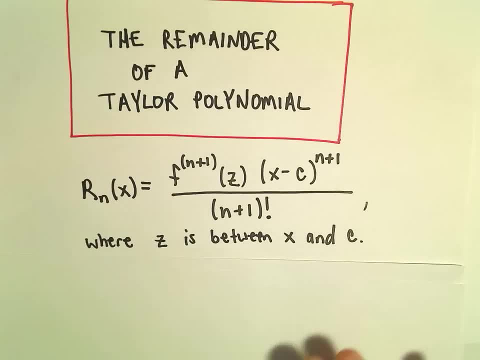 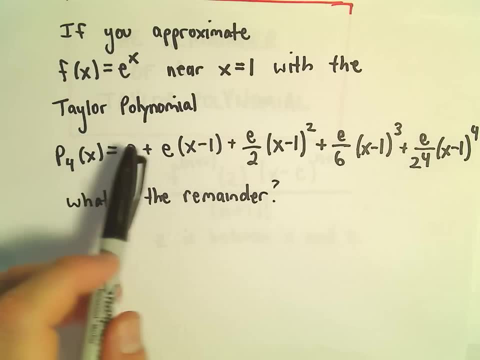 and then just plug in where we're centering it and calculate a few things. So let's look at an example here. So suppose we want to approximate the function e to the x near- x equals 1- with a polynomial, the Taylor polynomial. 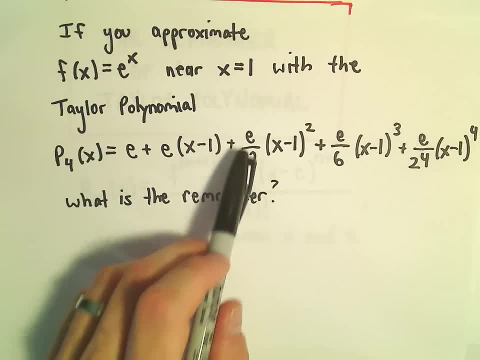 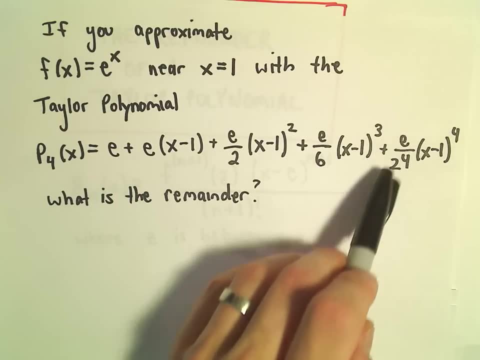 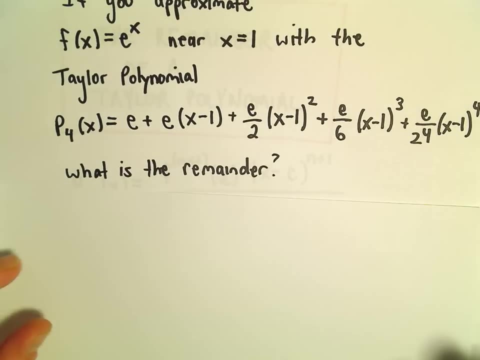 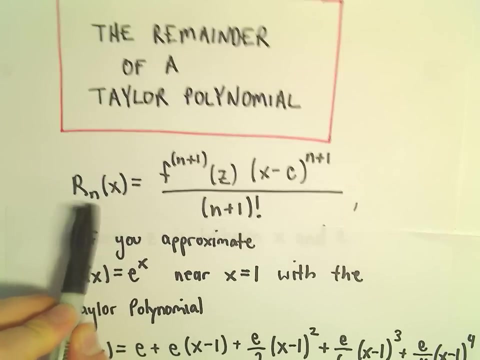 E plus e times x minus 1 plus, e over 2 times x minus 1 squared plus, e over 6 times x minus 1 cubed plus, e over 24 times x minus 1 to the fourth. Okay, so in our case so we're figuring out the remainder associated with a fourth-degree polynomial. 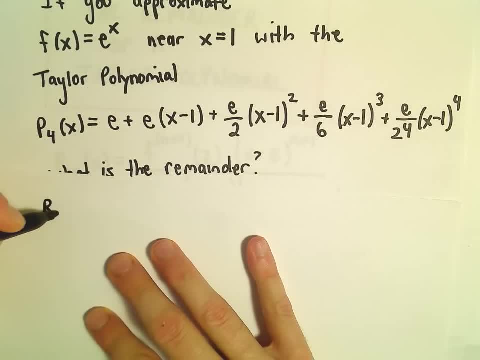 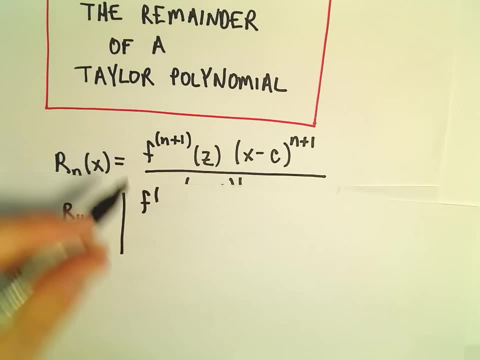 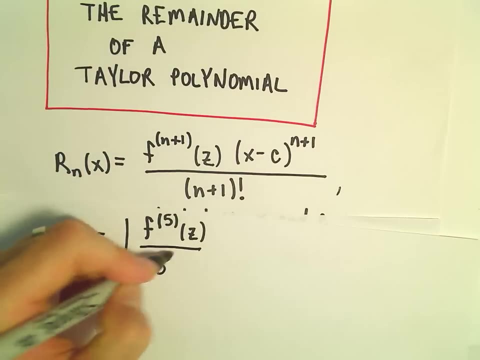 Okay, so we've gone out to degree 4.. So it says It says the remainder, and we need to put this in absolute value here. It says it'll be the well, the n plus 1, so the fifth derivative evaluated at z over well, again, we'll have 5 factorial. 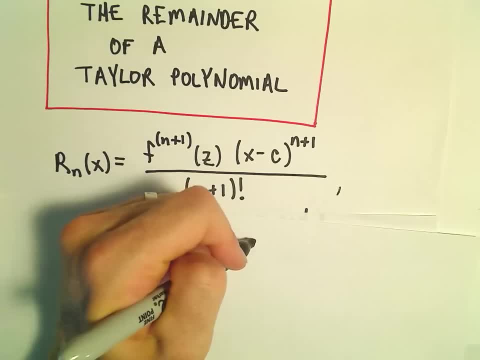 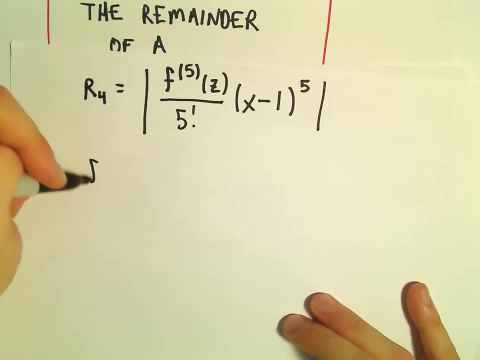 And then we'll take x minus where we're centering it, which for us is at positive 1. And then all of that will be raised to the fifth power. Well, in this case, our function f of x is just e to the x. 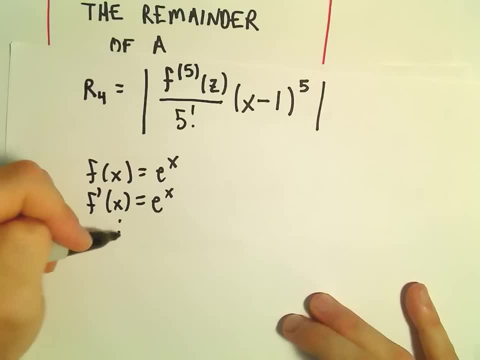 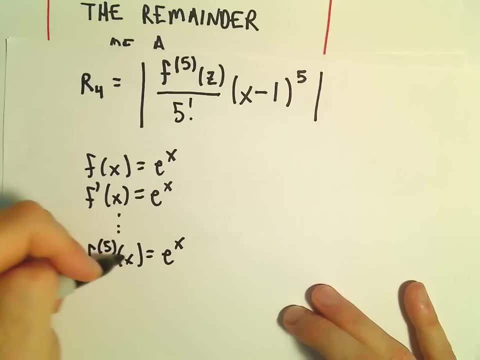 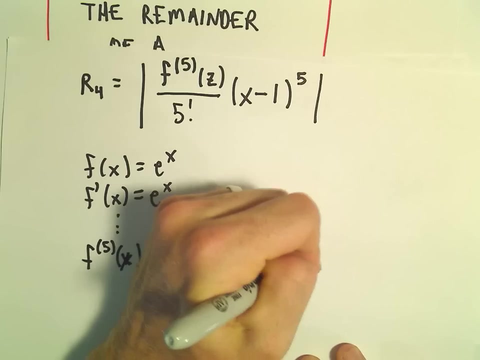 Well, all of the All of the derivatives for f of x are e to the x. So, eventually, the fifth derivative for x- well, that's also going to be e to the x. Well, that means the fifth derivative evaluated at z. well, that's simply going to equal e to the z. 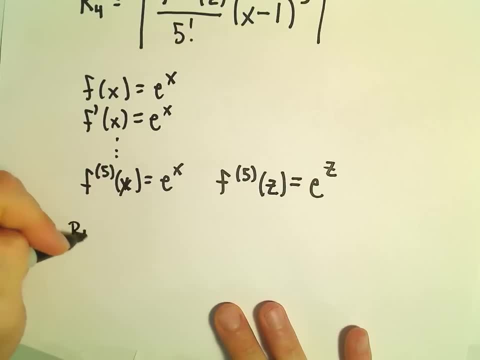 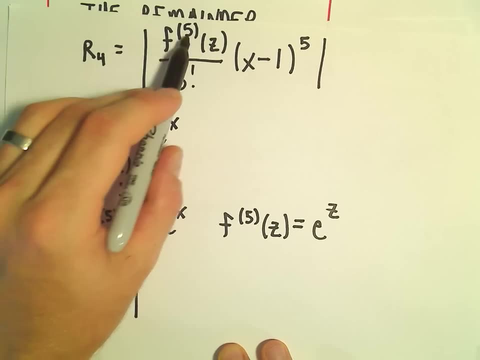 And now that's all we have to do is just simplify that and plug that in and simplify the expression. So again, the f of the fifth derivative, The derivative of our function evaluated at z, that's going to be e to the z. 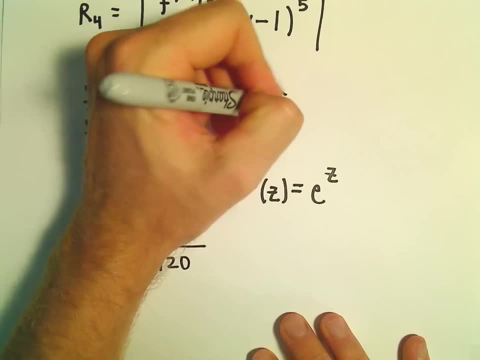 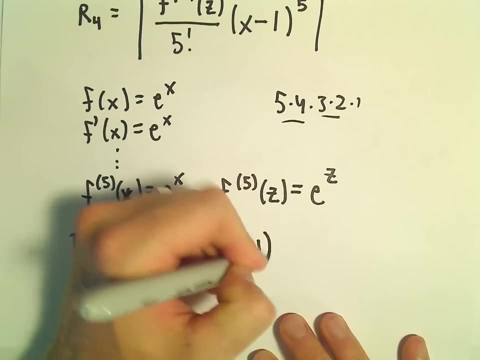 Let's see 5 factorial, I believe, that's 120.. So 5 times 4 times 3 times 2 times 1, that's 20.. And another 6, that's 120.. Then we'll have x minus 1 raised to the fifth power. 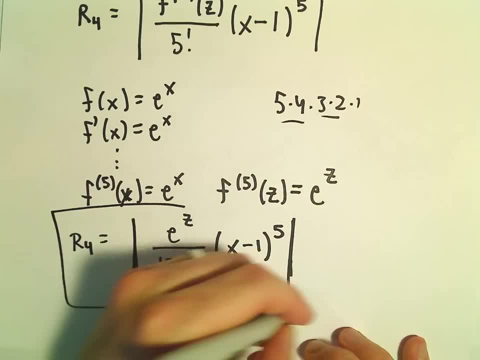 And that will now be an expression for our remainder.